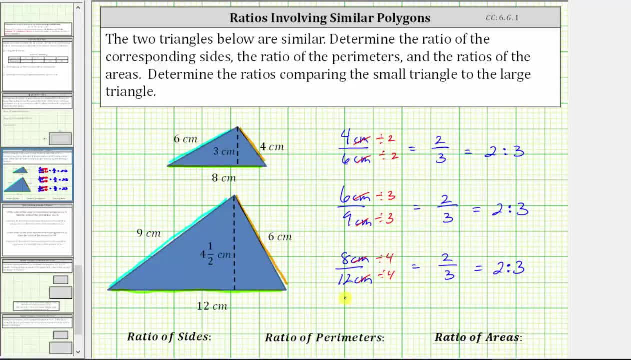 Once again giving us the ratio of two to three. The ratio of the corresponding sides is two to three. And now let's find the ratio of the perimeters. To find the perimeter, we sum the lengths of the sides, So the perimeter of the small triangle. 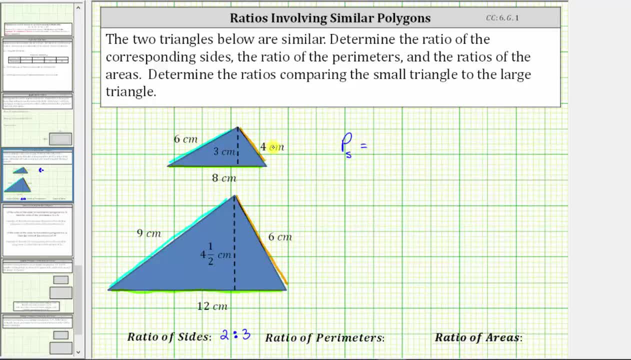 which we'll label P sub S, is equal to four centimeters plus six centimeters plus eight centimeters. Four plus six plus eight is 18.. The perimeter of the small triangle is 18 centimeters, And now we'll find the perimeter of the large triangle. 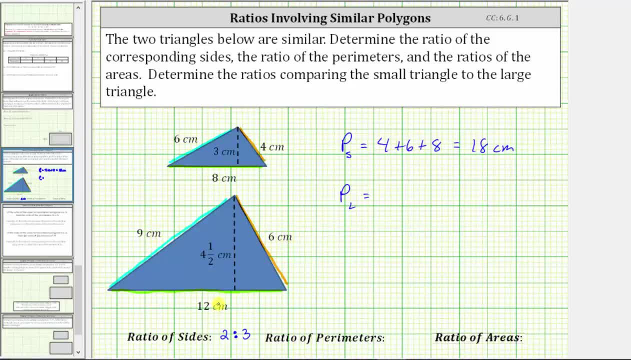 which is equal to six centimeters plus nine centimeters plus 12 centimeters. Six plus nine plus 12 is equal to 27.. The perimeter of the large triangle is 27 centimeters, Which means the ratio of the perimeters is 18 centimeters to 27 centimeters. 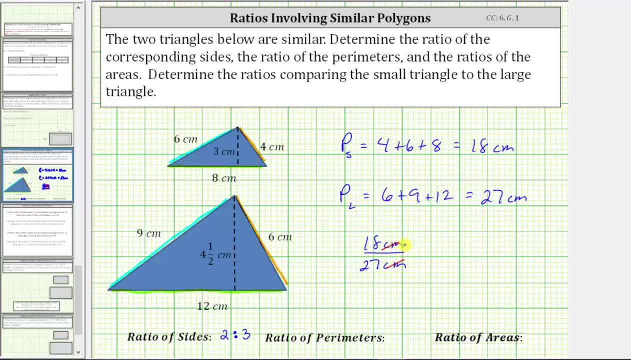 Again, the units of centimeters simplify out. The greatest common factor between 18 and 27 is nine. To simplify the ratio, we divide 18 by nine And 27 by nine. 18 divided by nine is two. 27 divided by nine is three. 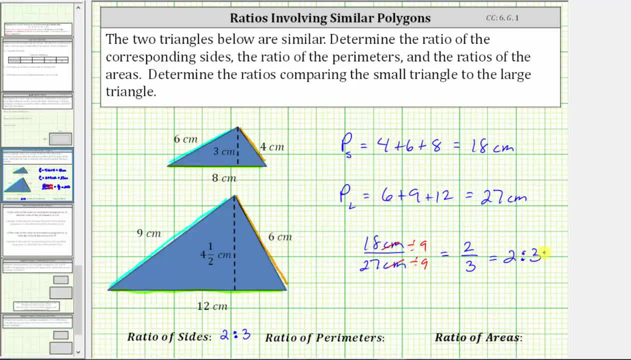 The ratio of the perimeters is the same as the ratio of the corresponding sides, which is two to three. Now we will determine the ratio of the areas. The area of a triangle is equal to one half base times height, So the area of the small triangle is equal to one half times. 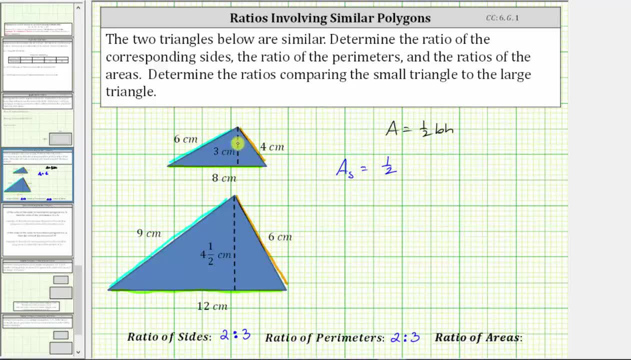 The area of the large triangle Is equal to one half base times height, a base of eight centimeters times the height of three centimeters. 1 1⁄2 times eight times three will give us the area of the small triangle. 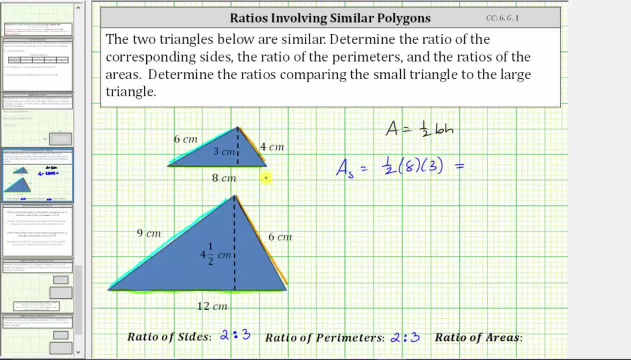 1 1⁄2 times eight is four. four times three is 12.. The area of the small triangle is 12 square centimeters, And now we'll find the area of the large triangle, which is 1 1⁄2 times the base of 12 centimeters. 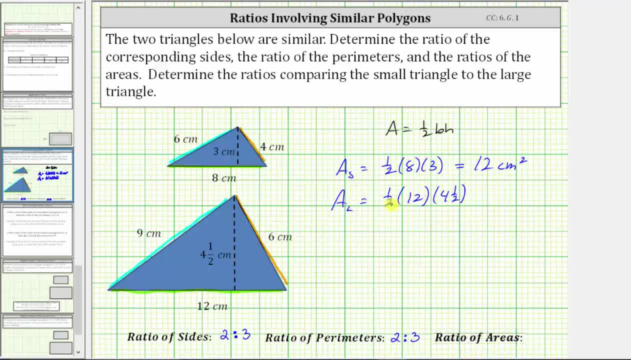 times the height of 4 1⁄2 centimeters. Multiplying 1 1⁄2 times 12 is six. The area is equal to six times 4 1⁄2.. Let's write six as a fraction, with a denominator of one. 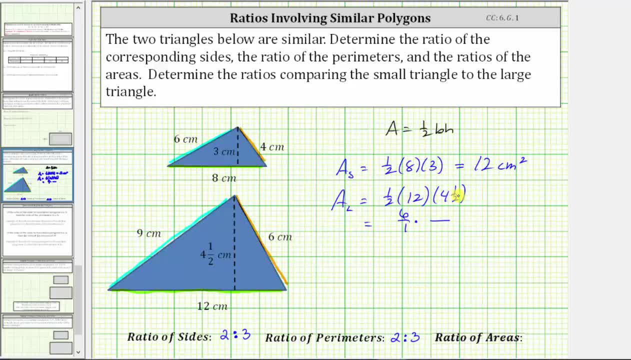 We'll write 4 1⁄2 as a improper fraction. The denominator remains two, The numerator is two times four plus one, which is nine. 4 1⁄2 is equal to 9 1⁄2.. 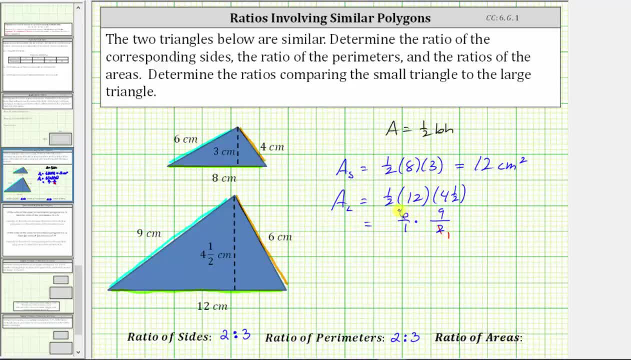 And now we simplify: before multiplying, There's one, two and two and three, twos and six. We now have three times nine, which is 27,. giving us an area of 27 square centimeters, which means the ratio of the areas. 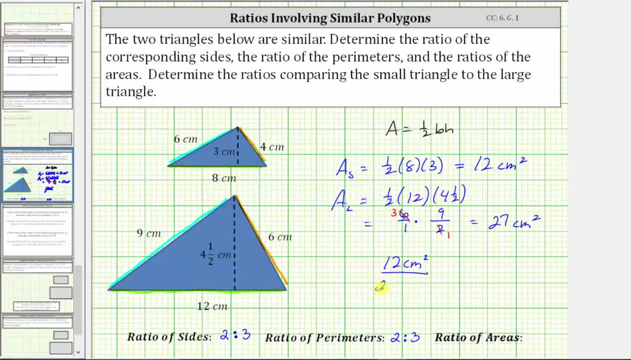 is 12 centimeters squared to 27 centimeters squared. The units of square centimeters simplifies out The greatest common factor between 12 and 27 is three. To simplify the ratio, we divide 12 by three and we get 1: 1⁄2.. 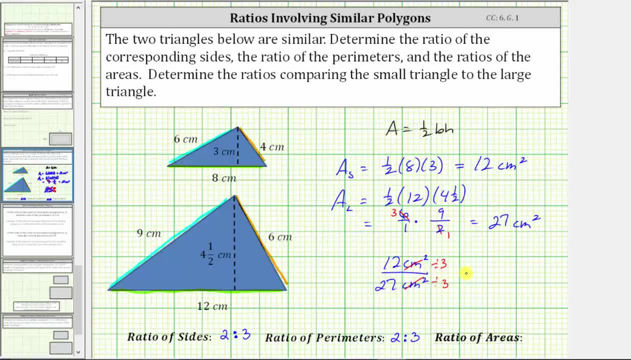 And we divide 27 by three, 12 divided by three is equal to four and 27 divided by three is nine. The ratio of the areas is not the same as the ratio of the sides and the ratio of the perimeters. The ratio of the areas is four to nine. 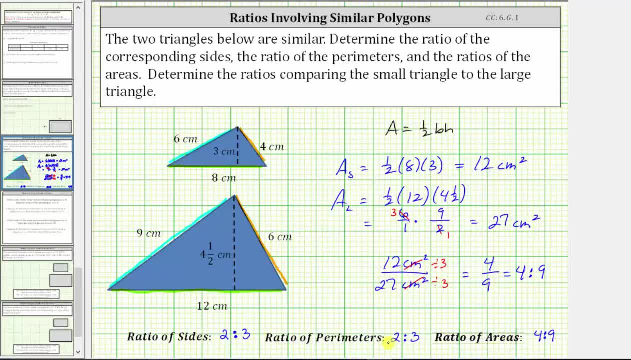 Notice how, if we begin with the ratio of the sides or the ratio of the perimeters, which is two to three, and then we square the two and we square the three, this does give us the ratio of the areas, which is four to nine. 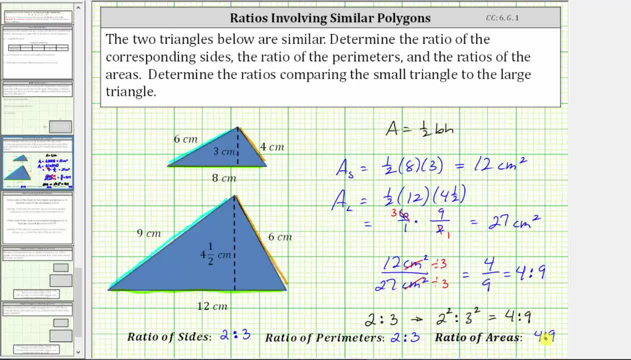 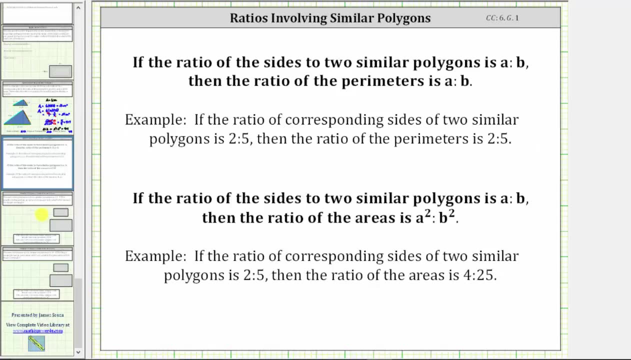 So it is true, the ratio of the areas is always the square of the ratio of the sides or the ratio of the perimeters, And this is not only true for similar triangles, it's true for all similar polygons. Let's summarize this. 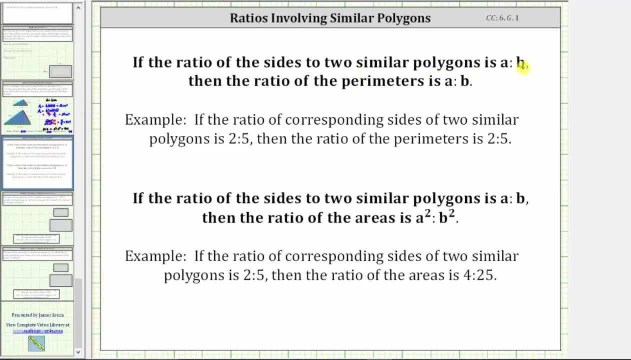 If the ratio of the sides of two similar polygons is a to b, then the ratio of the perimeters is also a to b. And here's an example: If the ratio of the sides of two similar polygons is a to b, then the ratio of the areas is a squared to b squared.